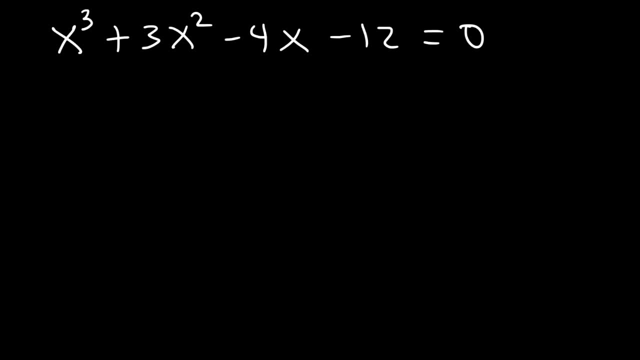 Now notice that the ratio of the first two coefficients is the same as the ratio of the last two. So, for example, 1 and 3 has the same ratio as negative 4 and negative 12.. Negative 12 divided by negative 4 is equal to 3, and 3 divided by 1 is 3.. 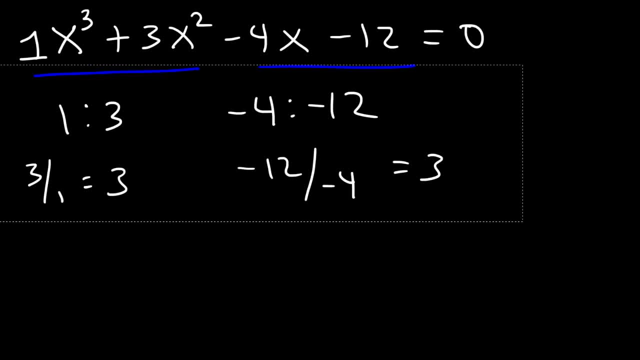 Whenever you see that you can factor by grouping, and in fact that's the best way, or the fastest way to get the answer. So let's take out the GCF. in the first two terms, The greatest common factor is X squared X cubed. divided by X squared is X. 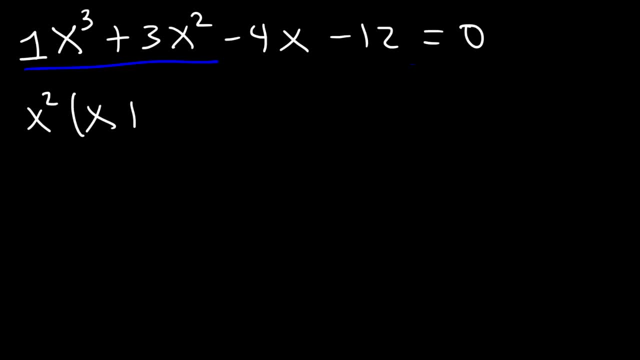 And 3x squared. divided by X squared is 3.. Now, in the last two terms, let's take out the GCF as well. The greatest common factor is negative 4.. Negative 4x divided by negative 4 is X. 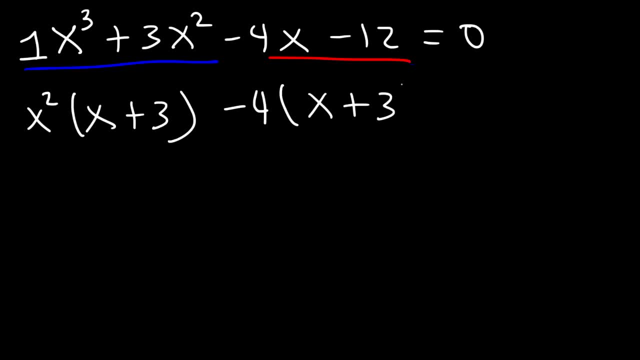 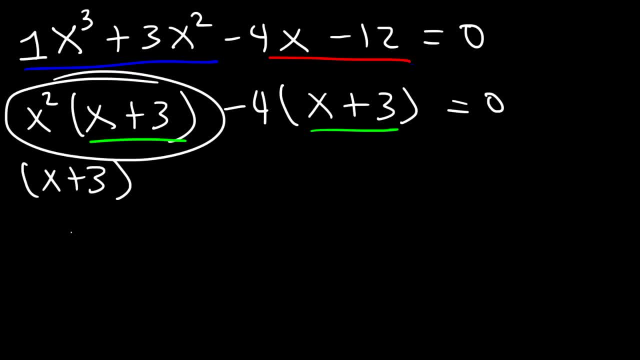 So let's take out X plus 3.. So this whole thing divided by X plus 3, is X squared, And this whole thing divided by X plus 3, is negative 4.. Now we're not done yet. 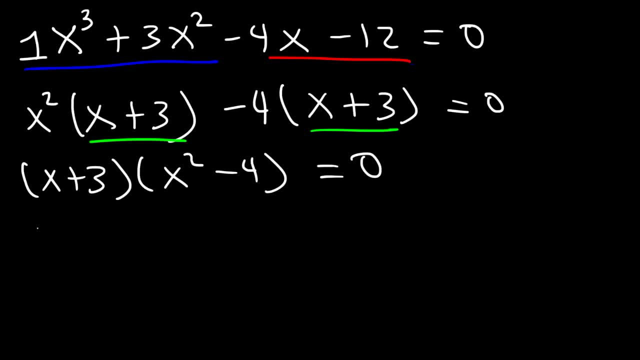 We can still factor X squared minus 4.. It's a difference of perfect squares. The square root of X squared is X. The square root of 4 is 2.. One is going to be positive and the other will be negative. So now the polynomial expression has been completely factored. 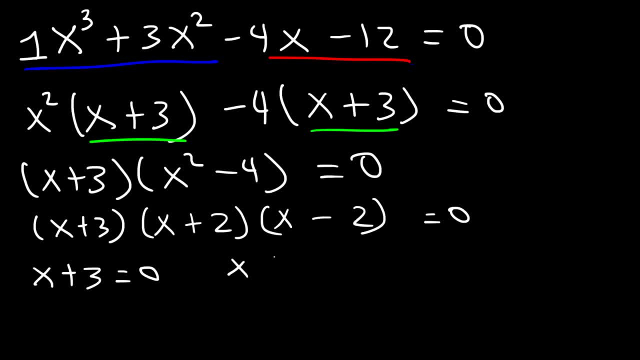 At this point, we can set each factor equal to zero, And so we're going to get three answers. So x is equal to negative 3,, it's equal to negative 2, and positive 2 as well. So that's how you can solve this particular polynomial equation. 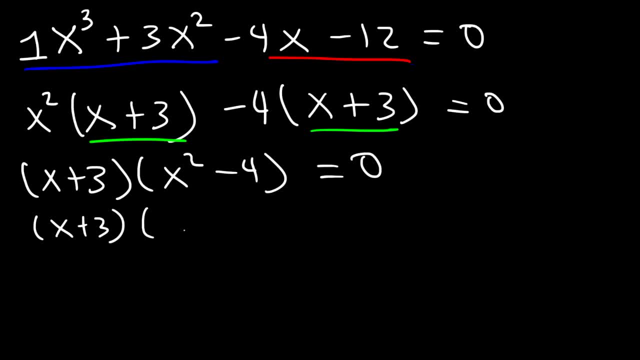 difference of perfect squares. The square root of x squared is x. The square root of 4 is 2.. One is going to be positive and the other will be negative. So now the polynomial expression has been completely factored. At this point we can. 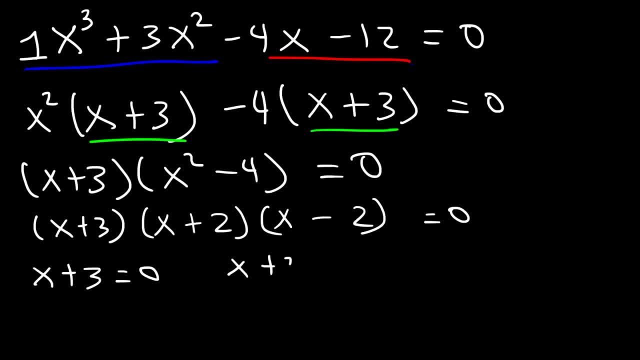 set each factor equal to zero, And so we're going to get three answers. So x is equal to negative 3. It's equal to negative 2 and positive 2 as well. So that's how you can solve this particular polynomial equation. 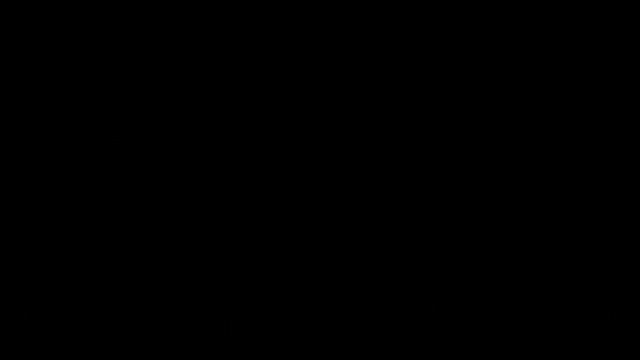 Now let's move on to our next example. So let's say that x to the fourth minus 5x, squared minus 36, is equal to zero. How can we solve this particular polynomial equation? Notice that this equation is reducible to a quadratic form, So we can factor it using. 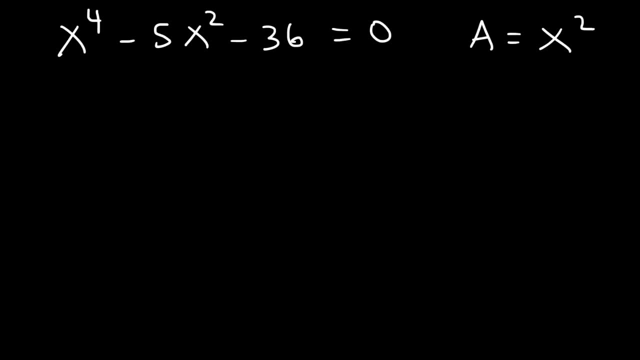 substitution. Let's say that a is equal to x squared. So that means that a squared squared is equal to x to the fourth. So let's replace x to the fourth with a squared and x squared with a. So now we have a trinomial with a leading coefficient of 1.. 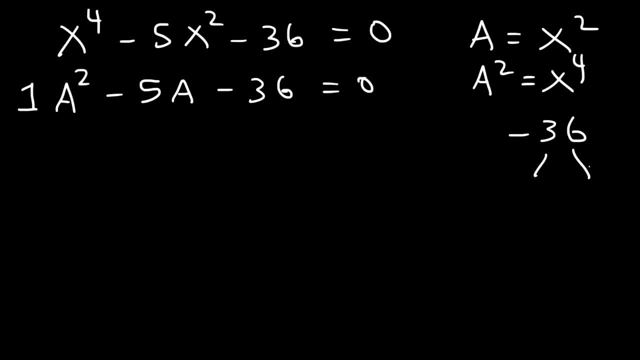 So what? two numbers multiply to negative 36 but add to negative 5? So this is going to be 9 and 4, but negative 9 and positive 4.. Negative 9 times 4 is negative 36, but negative 9 plus 4 is negative 5.. 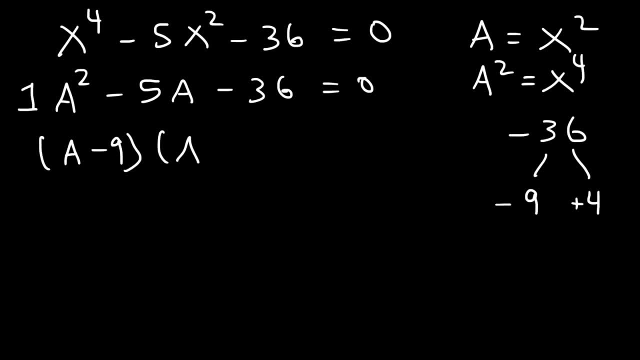 So to factor, it's going to be a minus 9 and a plus 4.. So at this point I'm going to replace a with x squared, So it's the same as x squared minus 9 times x squared plus 4.. Now you can factor x squared minus 9.. 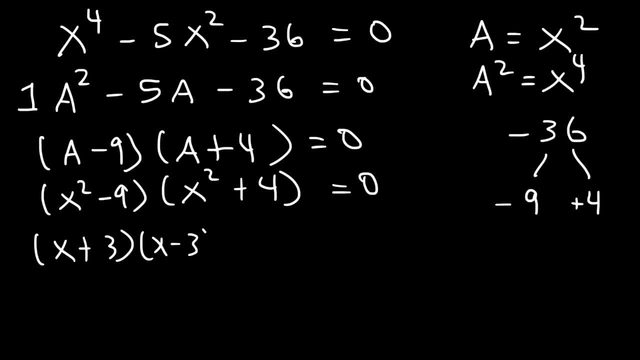 It's going to be x plus 3 and x minus 3 if you have a difference of perfect squares, If you have a sum of perfect squares, you can factor it using imaginary numbers. So it's going to be x plus 2i and x minus 2i. 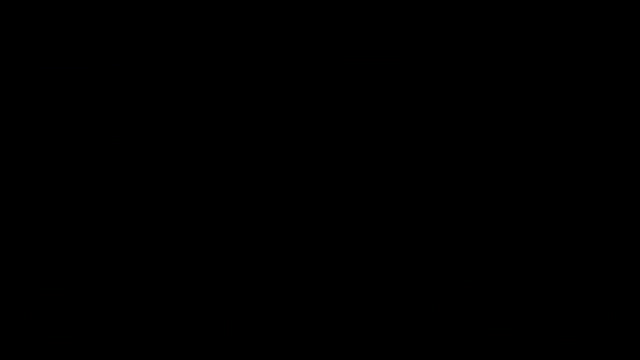 Now let's move on to our next example. So let's say that x to the 4th minus 5x, squared minus 36, is equal to zero. How can we solve this particular polynomial equation? Notice that this equation is reducible to a quadratic form. 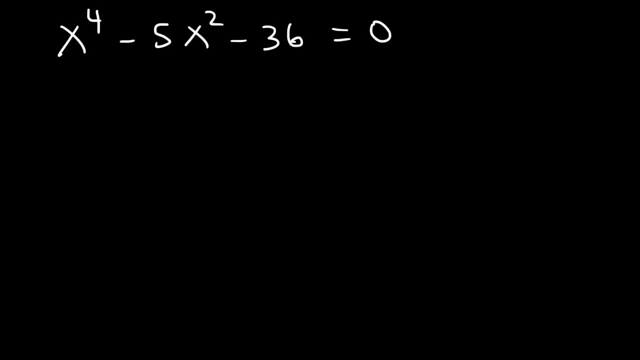 So we can factor it using substitution. Let's say that a is equal to x squared, So that means that a squared is equal to x to the 4th. So let's replace x to the 4th, x to the 4th with a squared and x squared with a. 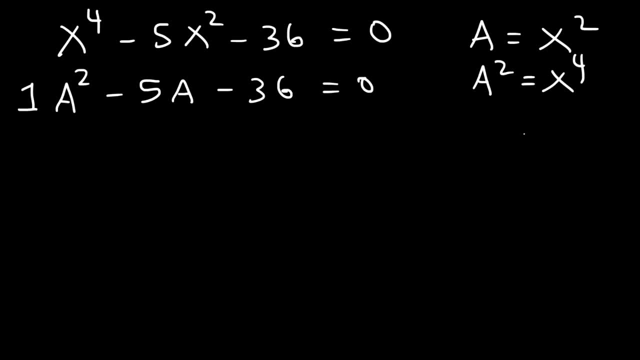 So now we have a trinomial with a leading coefficient of 1.. So what two numbers multiply to negative 36, but add to negative 5? So this is going to be 9 and 4, but negative 9 and positive 4.. 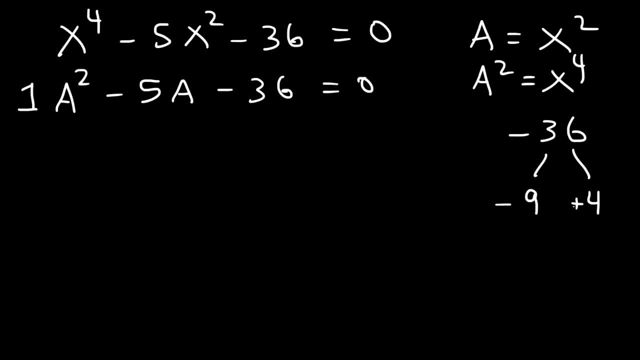 Negative 9 times 4 is negative 36, but negative 9 plus 4 is negative 5.. So to factor it, it's going to be a minus 9 and a plus 4.. Let's do that. So at this point I'm going to replace a with x squared. 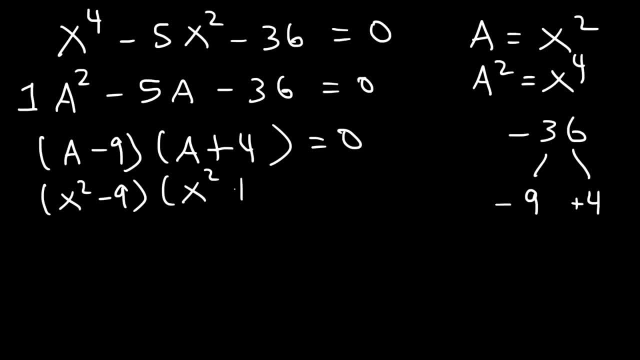 So it's the same as x squared minus 9 times x squared plus 4.. Now you can factor x squared minus 9.. It's going to be x plus 3 and x minus 3, if you have a difference of perfect squares. 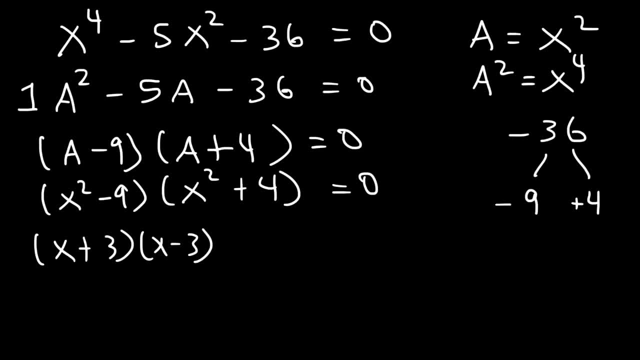 If you have a sum of perfect squares, you can factor it using imaginary numbers. So it's going to be x plus 2i and x minus 2i. Let's do that. So, because it's a polynomial of degree 4, there's going to be four answers. 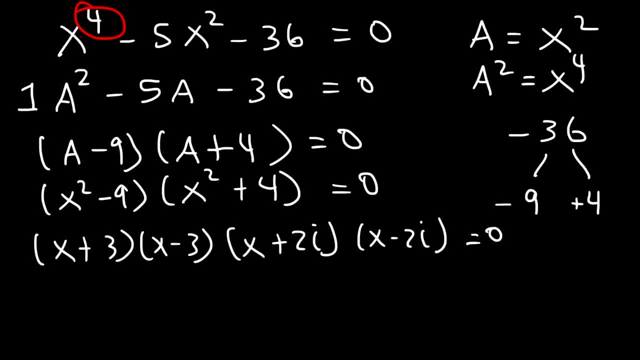 But in this case two of them are real numbers and the other two are imaginary numbers. So x is equal to negative 3, 3, negative 2i and 2i. So you can write it this way: x is equal to plus or minus 3, or plus or minus 2i. 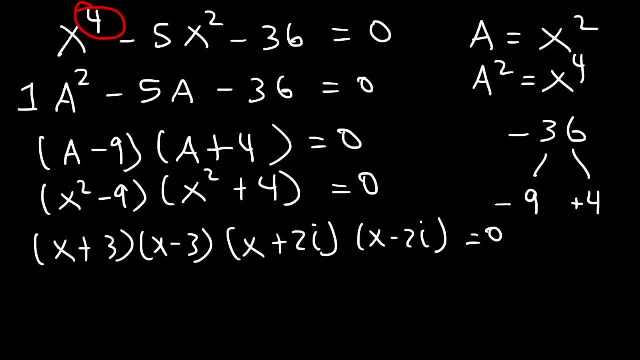 So, because it's a polynomial of degree 4, there's going to be four answers, but in this case two of them are real numbers and the other two are imaginary numbers. So x is equal to negative 3, 3, negative 2i and 2i. 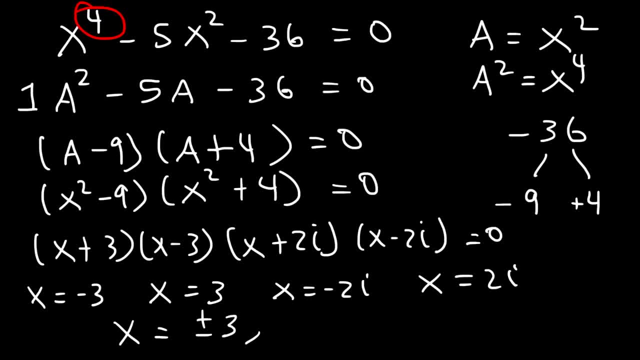 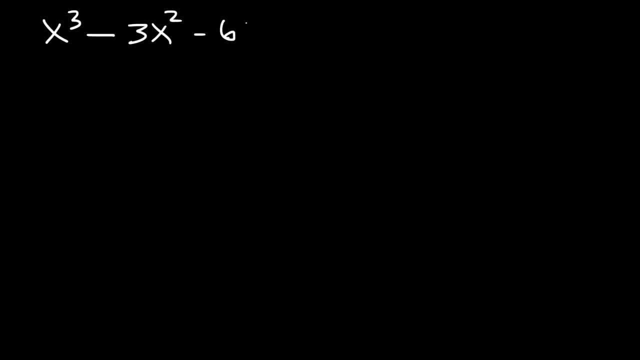 So you can write it this way: x is equal to plus or minus 3.. Or x is equal to minus 2i. So those are the four answers for this problem. Let's try this: one: x cubed minus 3x squared minus 6x plus 8 is equal to 0.. 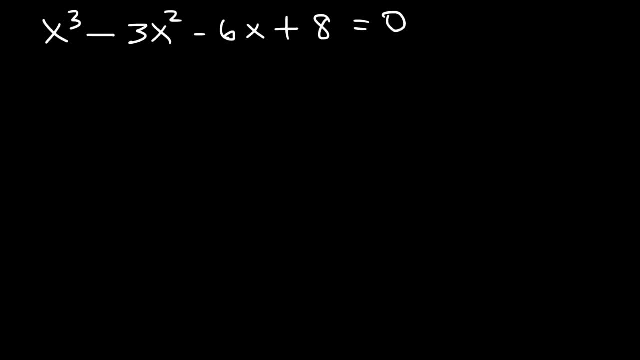 Find all the zeros of the function, Go ahead and solve for the value of x. Now we can't factor by grouping because the first two terms do not have the same ratio as the last two. Negative 3 divided by 1 is not the same as 8 divided by negative 6, which reduces to negative. 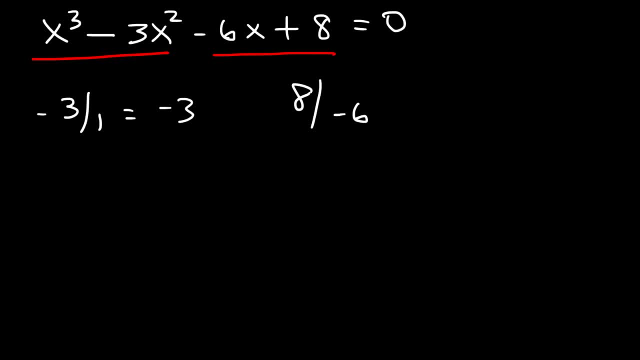 four thirds. So we can't factor by grouping and we can't reduce it to quadratic form. So the last method that we can use is we need to list all the possible rational zeros using the rational zero theorem and then use synthetic division to find out the other zeros. 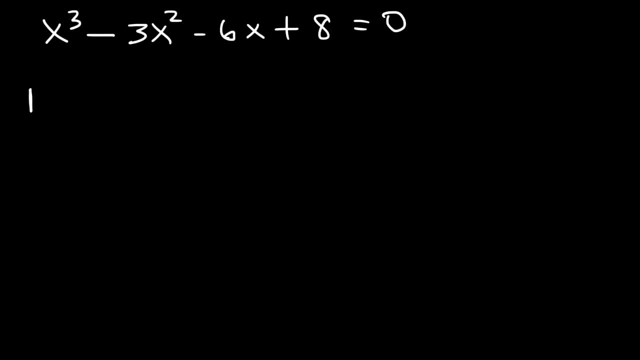 So p is equal to 0.. 0 is equal to 0.. 0 is equal to negative. 2i 0 is equal to 0.. 0 is equal to negative. 2i 0 is equal to 0.. 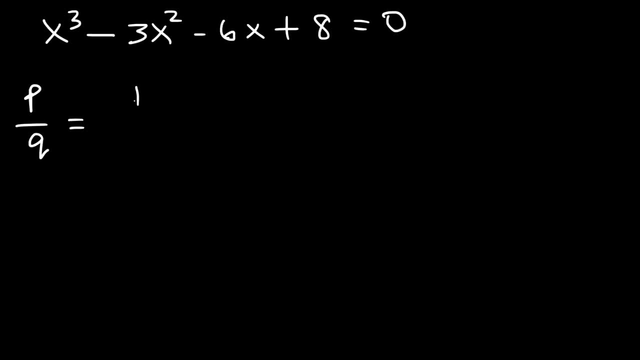 Q represents the factors of the constant term 8.. So factors of 8 are 1,, 2,, 4, and 8.. Q represents the factors of 1, the lean coefficient. So let's evaluate the function at: x equals 1.. 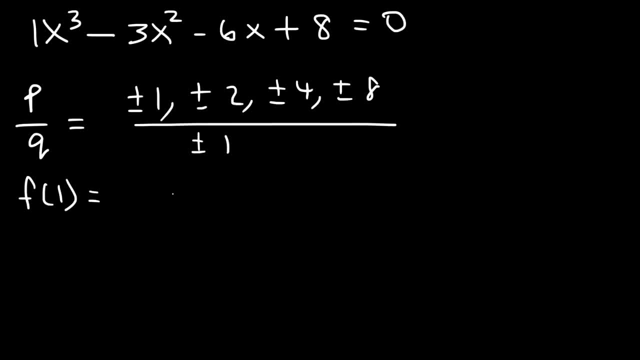 Let's see if that is a possible answer. 1 to the 3rd minus 3 times 1, squared minus 6 times 1 plus 8.. Let's see if it's equal to 0.. So 1 to the 3rd is 1.. 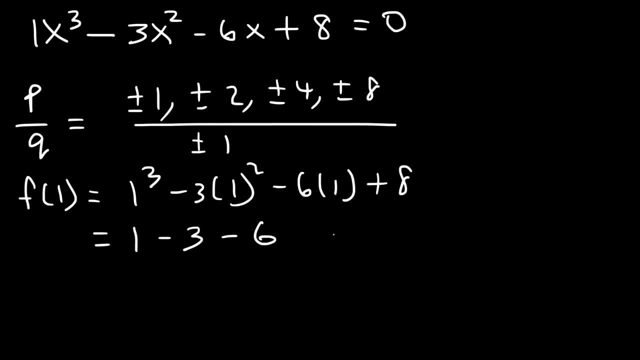 3 times 1, squared is 3.. And then we have 6 plus 8.. So 1 minus 3 is negative 2. And negative 2 minus 6 is negative 8.. Negative 8 plus 8 is equal to 0.. 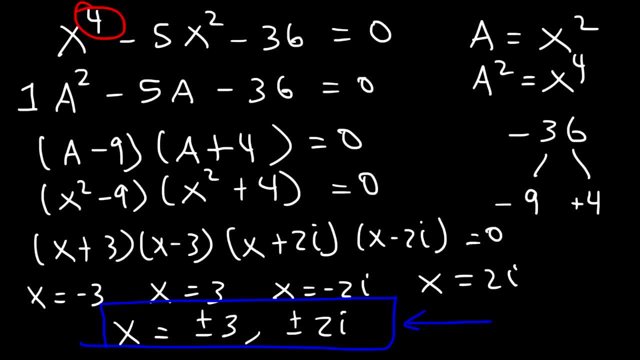 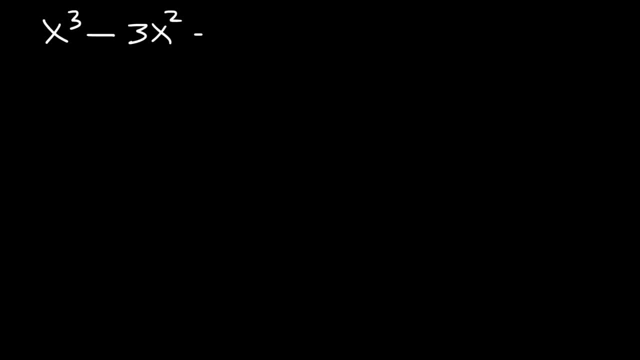 So those are the four answers For this problem. Let's try this: one x cubed minus 3x. squared minus 6x plus 8 is equal to 0.. Find all the zeros of the function. Go ahead and solve for the value of x. 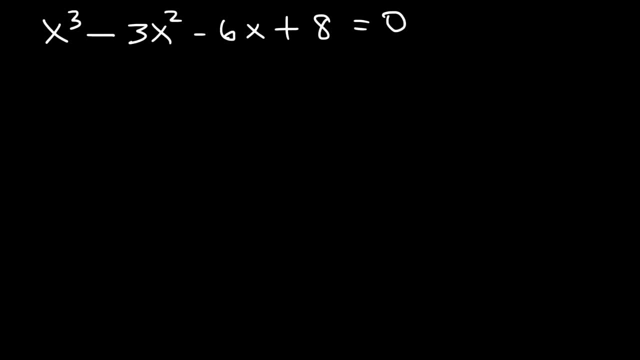 Now we can't factor by grouping, because the first two terms do not have the same ratio as the last two. Negative 3 divided by 1 is not the same as 8.. Negative 3 divided by 1 is not the same as 8, divided by negative 6,, which reduces to negative 4 thirds. 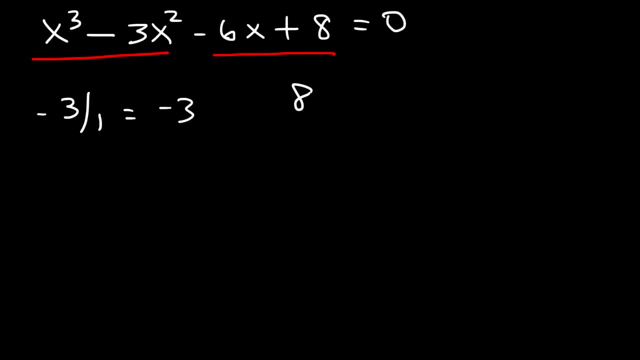 So we can't factor by grouping and we can't reduce it to quadratic form. So the last method that we can use is we need to list all the possible rational zeros using the rational zero theorem and then use synthetic division to find out the other zeros. 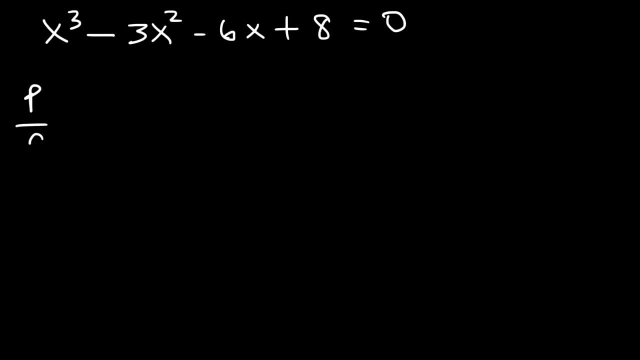 So p represents the factors of the constant term 8.. So factors of 8 are 1,, 2,, 4, and 8.. Q represents the factors of 1, the lean coefficient. So let's evaluate the function at: x equals 1.. 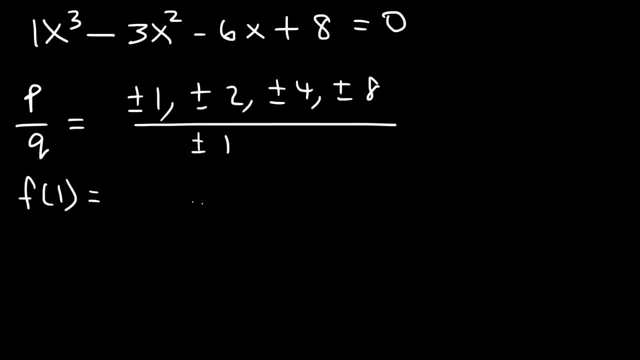 Let's see if that is a possible answer: 1 to the third minus 3 times 1 squared, minus 6 times 1 plus 8.. Let's see if it's equal to 0.. So 1 to the third is 1,, 3 times 1 squared is 3, and then we have 6 plus 8.. 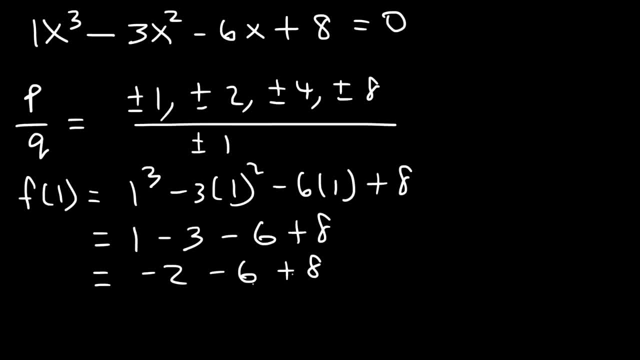 So 1 minus 3 is negative 2, and negative 2 minus 6 is negative 8.. Negative 8 plus 8 is equal to 0. Because it's equal to 0, that means that this is one of the answers. 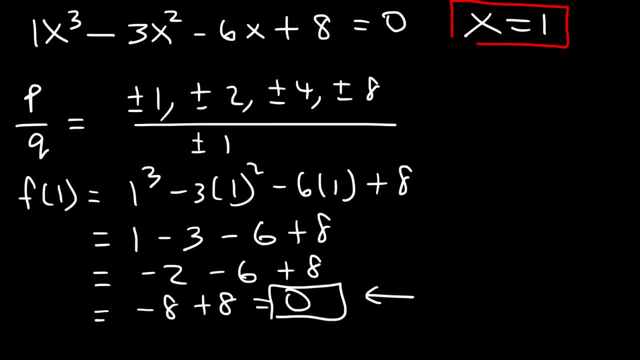 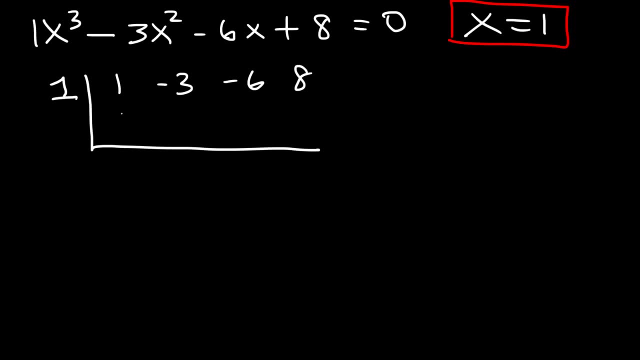 x is equal to 1.. Now let's find the other answers. So let's use synthetic division. The coefficients are 1, negative 3, negative 6, and 8.. So let's bring down the 1.. 1 times 1 is 1.. 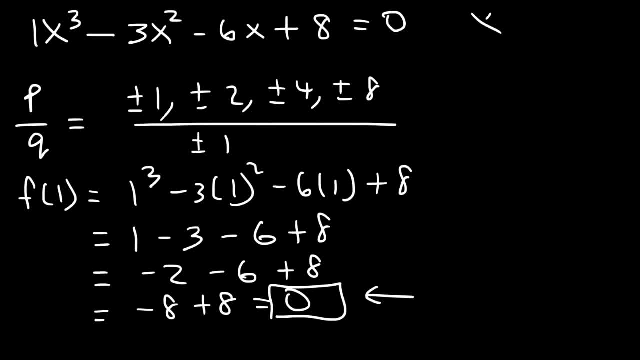 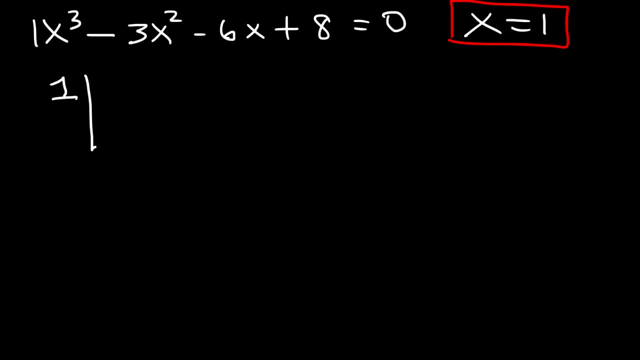 Because it's equal to 0, that means that this is one of the answers. x is equal to 1.. Now let's find the other answers, So let's use synthetic division. The coefficients are 1, negative, 3, negative, 6, and 8.. 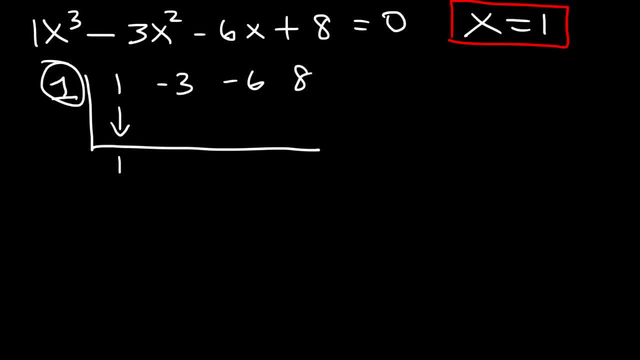 So let's bring down the 1.. 1 times 1 is 1. Negative 3 plus 1 is negative 2. And then 1 times negative: 2 is negative 2. Negative 6 plus negative 2 is negative 8.. 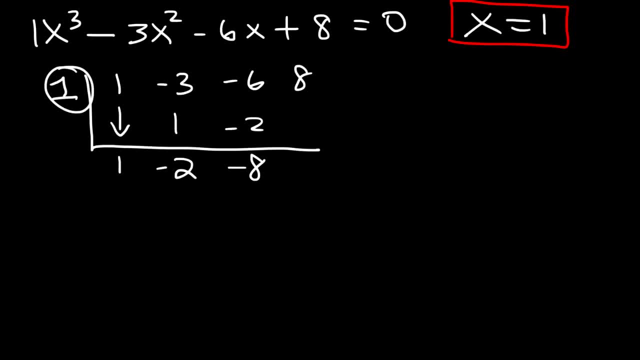 And then 1 times negative 8 is Negative 8. And 8 plus negative 8 is 0.. If this is not a 0, then a mistake occurred. So this is going to be 1x squared, which is 1 degree lower than this one. 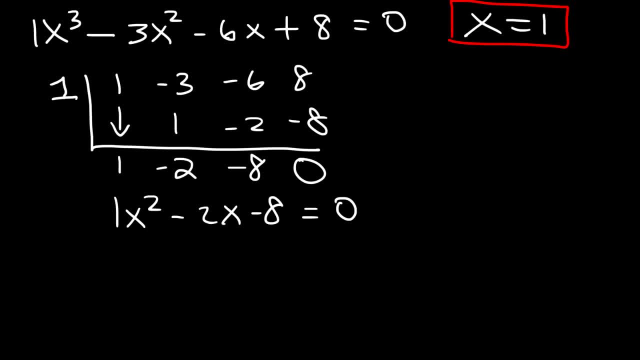 minus 2x minus 8.. And let's set that equal to 0.. Now let's see if we can factor this expression: Two numbers that multiply to 8 but add to the middle coefficient of negative 2 are going to be negative 4 and positive 2.. 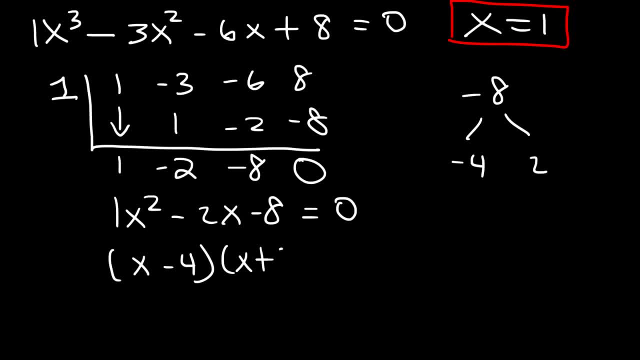 So to factor it, it's going to be x minus 4.. Times x plus 2.. So x is equal to 4 and negative 2.. So we have three real solutions: 4,, negative 2, and 1.. 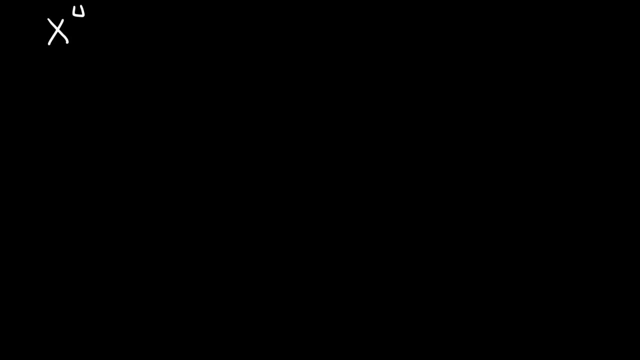 Here's another problem that we could try: x to the fourth power minus 7x cubed, plus 7x squared, plus 35x minus 60.. Go ahead and solve this particular polynomial equation So using the rational zero theorem. the factors of 60 are going to be: 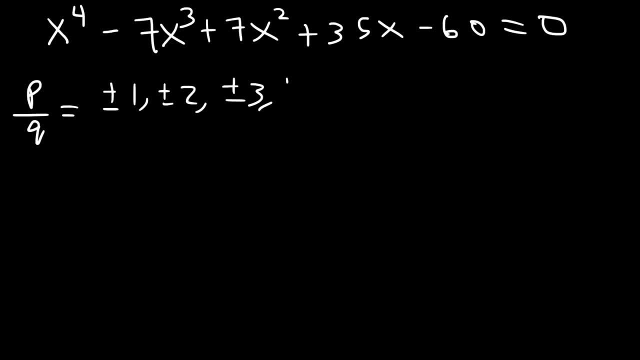 1,, 2,, 3,, 4,, 5,, 6,, 7 and 8 doesn't go into 60,, but 10 goes into it, 12,, 15,, 30, and 60, and 20 as well. 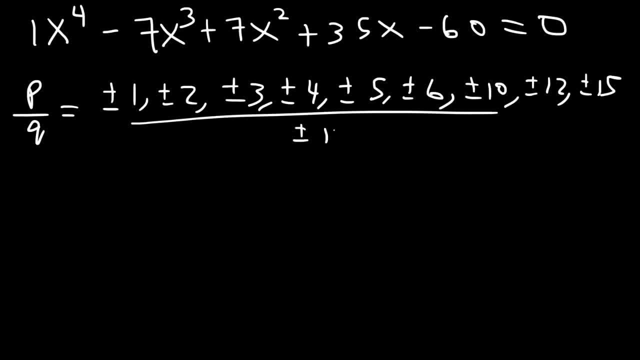 And then the leading coefficient is 1.. So there's a lot of factors, But let's start with 1.. Let's see if f of 1 is equal to 0. So that's going to be 1 to the fourth power. 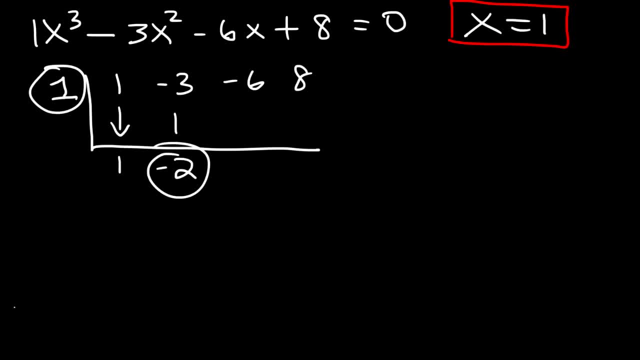 Negative 3 plus 1 is negative 2.. And then 1 times negative 2 is negative 2.. Negative 6 plus negative 2 is negative 8.. And then 1 times negative 8 is negative 8.. And 8 plus negative 8 is 0.. 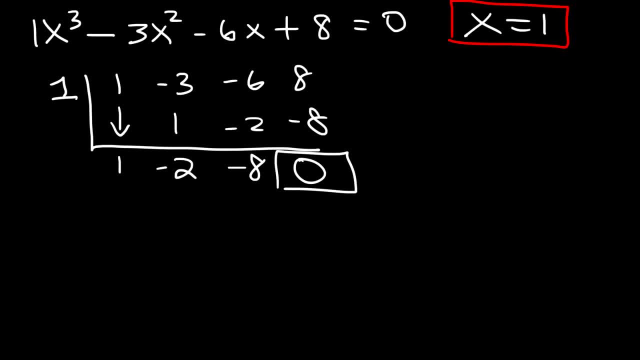 If this is not a 0,, then A mistake occurred. So this is going to be 1x squared, which is 1 degree lower than this one minus 2x minus 8.. And let's set that equal to 0.. 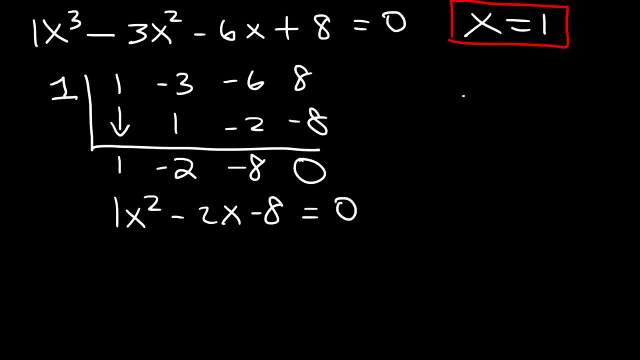 Now let's see if we can factor this expression. Two numbers that multiply to 8 but add to the middle coefficient of negative 2 are going to be negative 4 and positive 2.. So to factor it, it's going to be x minus 4 times x plus 2.. 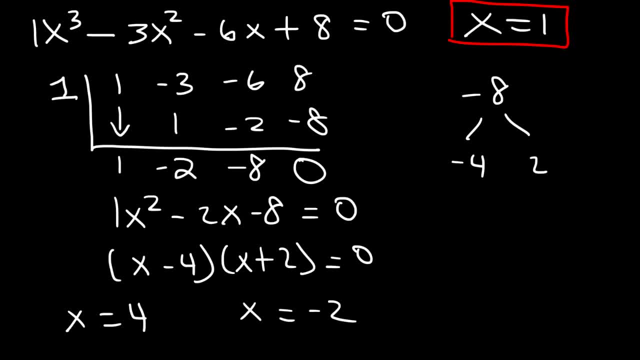 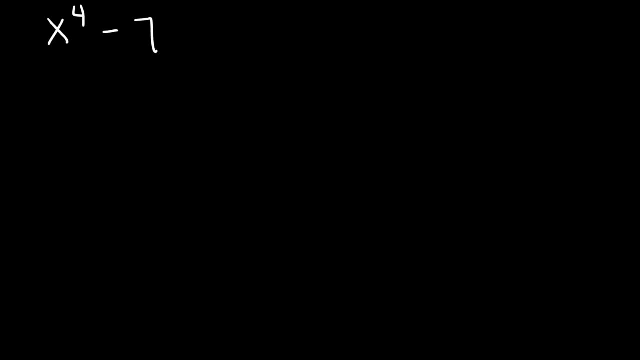 So x is equal to 4.. And negative 2.. So we have three real solutions: 4, negative 2, and 1.. Here's another problem that we could try: x to the fourth power minus 7x cubed, plus 7x squared, plus 35x, minus 60.. 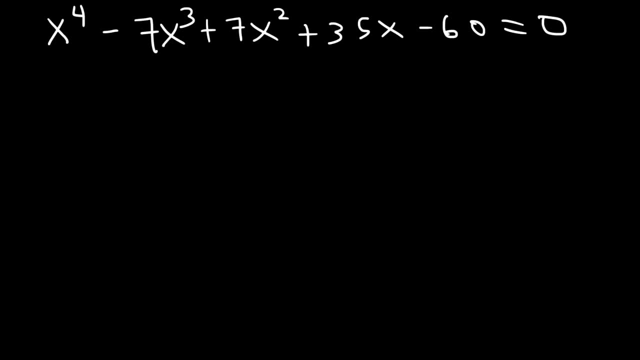 Go ahead and solve this particular polynomial equation. So use Using the rational zero theorem. the factors of 60 are going to be 1,, 2,, 3,, 4,, 5,, 6,, 7,. 8 doesn't go into 60, but 10 goes into it, 12,, 15,, 30, and 60, and 20 as well. 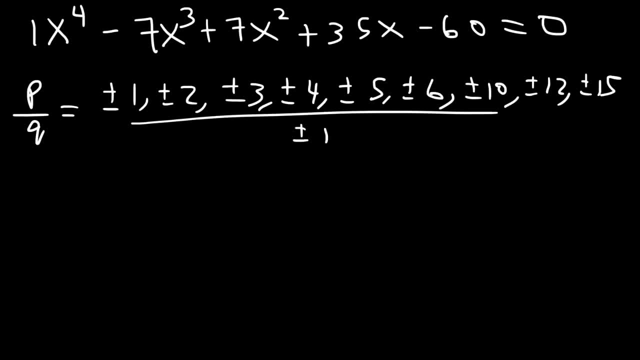 And then the leading coefficient is 1.. So there's a lot of factors, But let's start with 1.. Let's see if f of 1 is equal to 0. So that's going to be 1 to the fourth power minus 7 times 1 cubed plus 7 times 1 squared, plus 35 times 1 minus 60.. 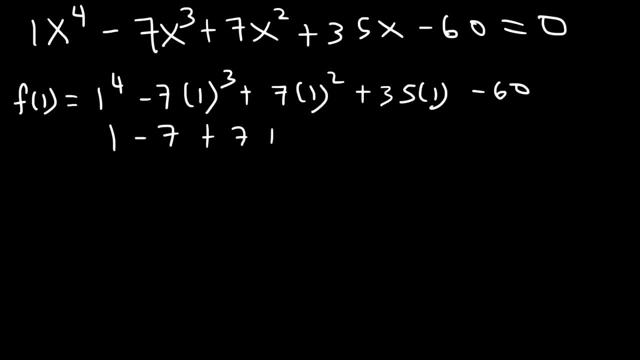 So this is going to be 1 minus 7 plus 7 plus 35 minus 60.. Negative 7 plus 7 is 0.. And 35 minus 60 is negative 25.. So negative 24 is not equal to 0.. 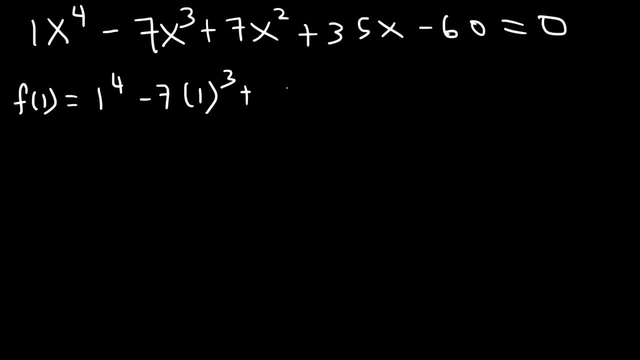 minus 7 times 1 cubed, plus 7 times 1 squared, plus 35 times 1 minus 60.. So this is going to be 1 minus 7 plus 7 plus 35 minus 60.. Negative: 7 plus 7 is 0.. 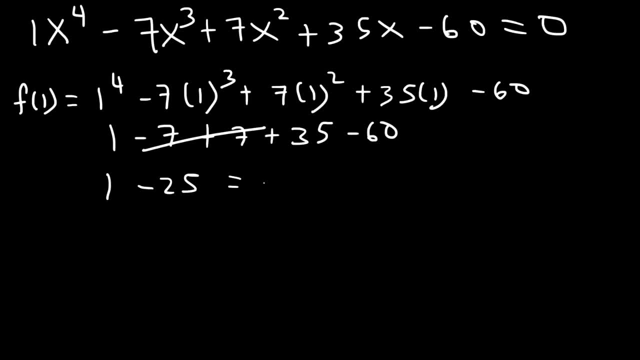 And 35 minus 60 is negative 25.. So negative 24 is not equal to 0. So this doesn't work. Let's try the next number, 2.. So it's going to be 2 to the fourth minus 7 times 2 to the third. 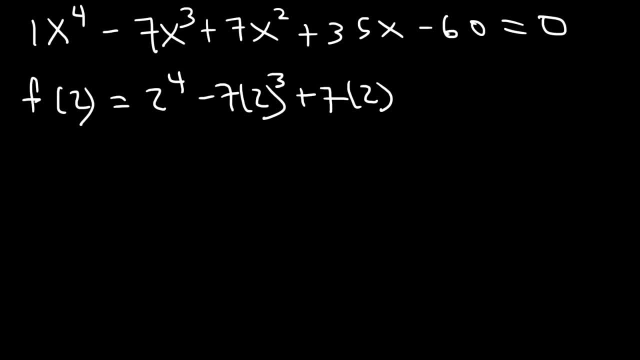 plus 7 times 2, squared plus 35 times 2 minus 60.. So 2 to the fourth, that's 2 times 2 times 2 times 2.. 2 times 2 is 4 times 2 is 8, times 2 is 16.. 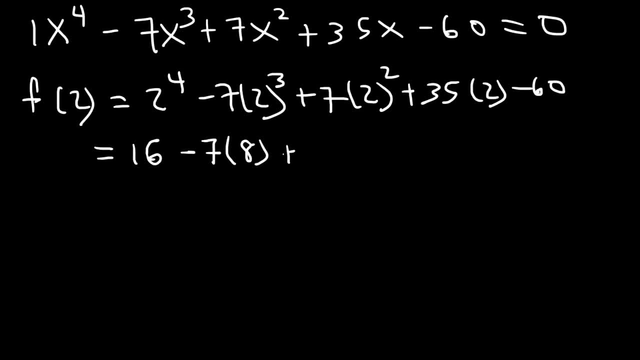 And then 2 to the third is 8.. 2 squared is 4.. 35 times 2 is 70.. And then 7 times 8 is 56.. 7 times 4 is 27.. That's 28.. 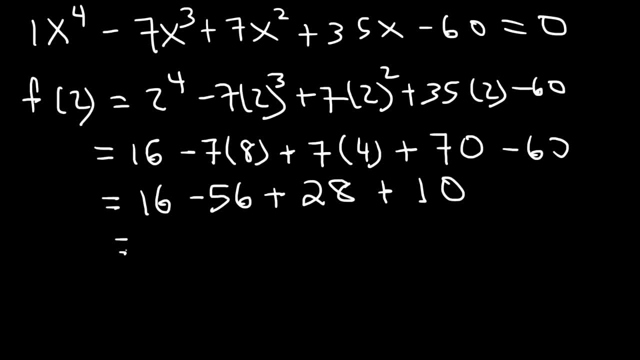 And 70 minus 60 is 10.. Now 16 minus 56,, that's negative 40. And 28 plus 10 is 38. Negative 40 plus 38 is negative 2, which is not 0. So that doesn't work either. 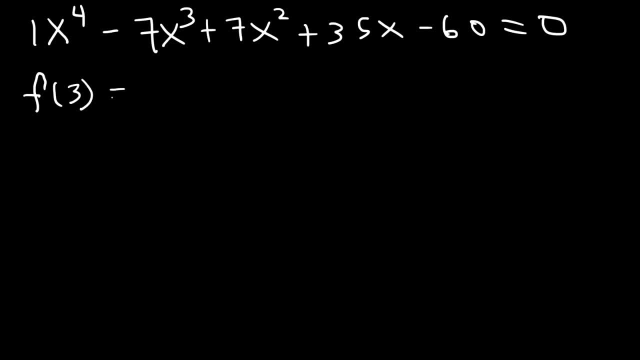 Now let's try 3.. So 3 to the fourth minus 7 times 3 to the third plus 7 times 3, squared plus 35 times 3 minus 60. Let's see if this gives us a 0.. 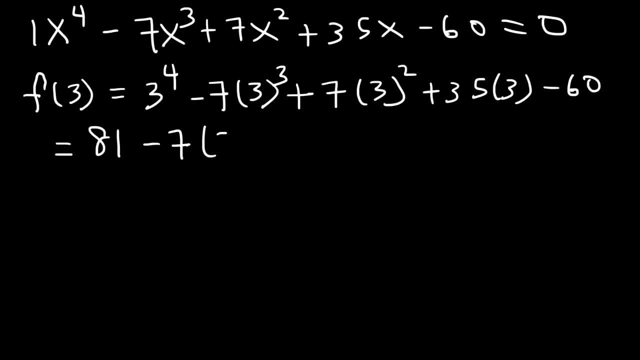 3 to the fourth, power is 81.. 3 to the third is 27.. And 3 squared is 9.. Now 35 times 3.. 30 times 3 is 90.. 3 times 5 is 15.. 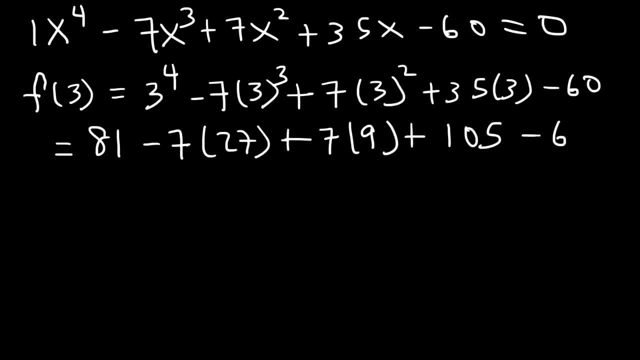 90 and 15 is 105.. Now 7 times 27.. 7 times 20 is 140.. 7 times 7 is 49.. So 140 and 49, that's going to be 189.. 7 times 9 is 63.. 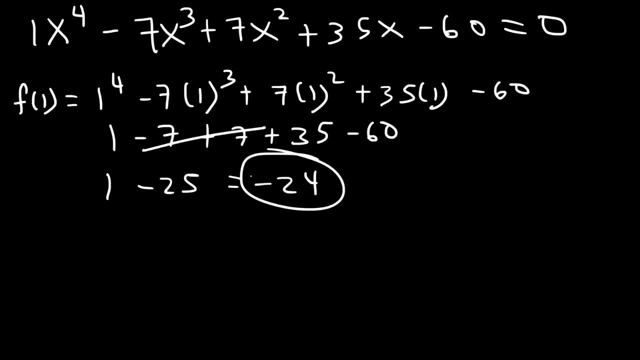 So This doesn't work, Let's try the next number, 2.. So it's going to be 2 to the fourth minus 7 times 2 to the third, plus 7 times 2 squared plus 35 times 2 minus 60.. 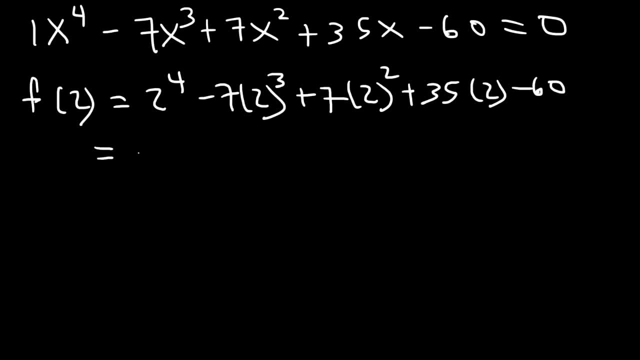 So 2 to the fourth, that's 2 times 2 times 2 times 2.. 2 times 2 is 4.. 4 times 2 is 8.. Times 2 is 16.. And then 2 to the third is 8.. 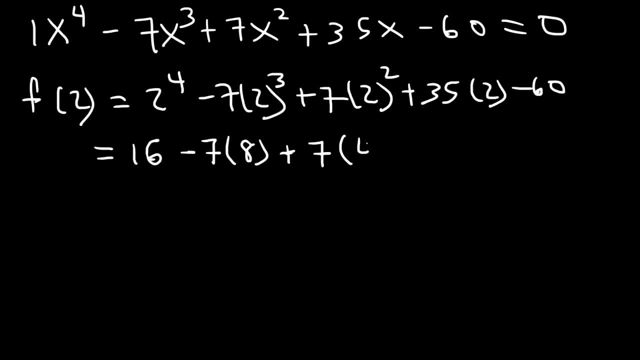 2 squared is 4.. 4.. 35 times 2 is 70.. And then 7 times 8 is 56.. 7 times 4 is 28.. And 70 minus 60 is 10.. Now 16.. 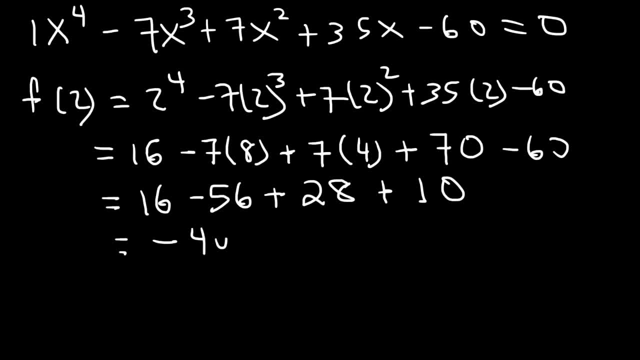 16 minus 56, that's negative 40. And 28 plus 10 is 38.. Negative 40 plus 38 is negative 2, which is not 0. So that doesn't work either. Now let's try 3.. 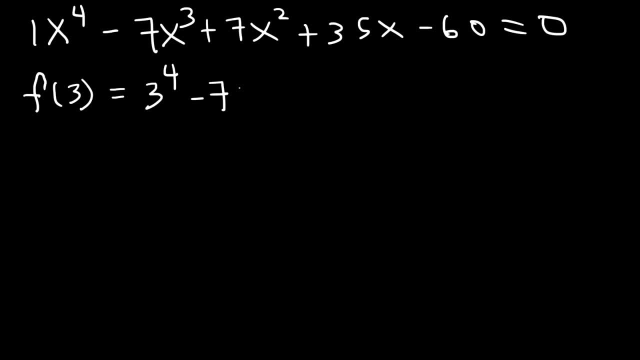 So 3 to the fourth, power minus 7 times 3 to the third, 3 to the third Plus 7 times 3 squared plus 35 times 3 minus 60.. Let's see if this gives us a 0.. 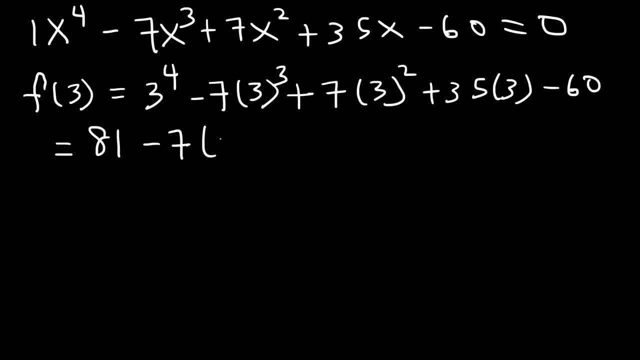 3 to the fourth, power is 81.. 3 to the third is 27.. And 3 squared is 9.. Now 35 times 3.. 30 times 3 is 90.. 3 times 5 is 15.. 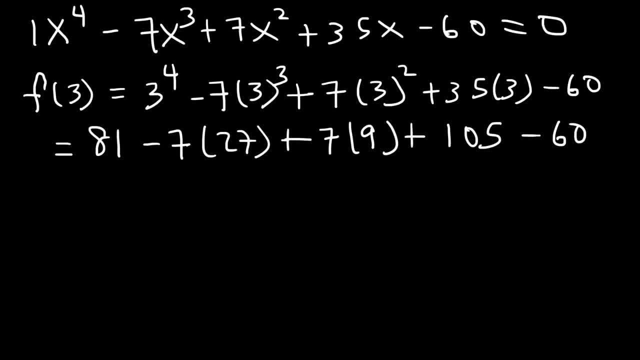 90 and 15 is 105.. Now 7 times 27.. 7 times 20 is 140.. 7 times 7 is 49.. So 140 and 49, that's going to be 189.. 7 times 9 is 63.. 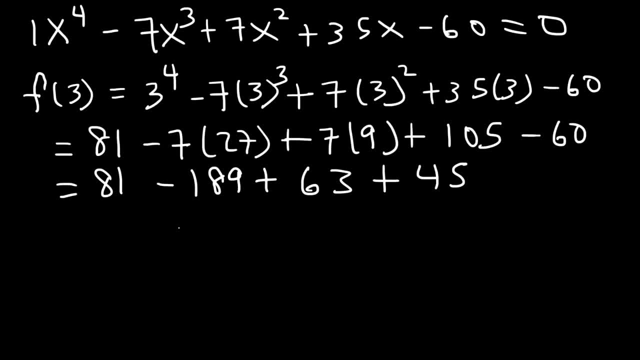 And 105 minus 60 is 45. So 81 minus 189, that's going to be negative 108. And 63 plus 45 is positive 108.. So this adds up to 0, which means x is equal to 3.. 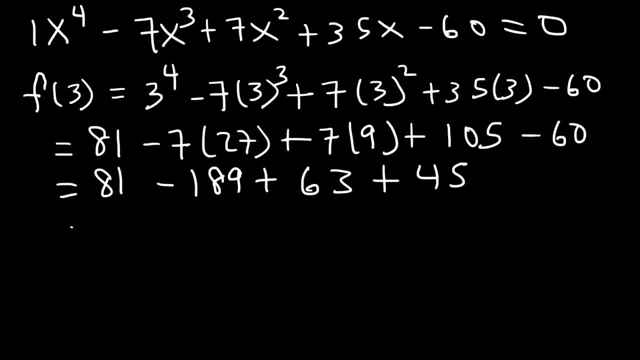 And 105 minus 60 is 45. So 81 minus 189, that's going to be negative 108. And 63 plus 45 is positive 108. So this adds up to 0. Which means X is equal to 3.. 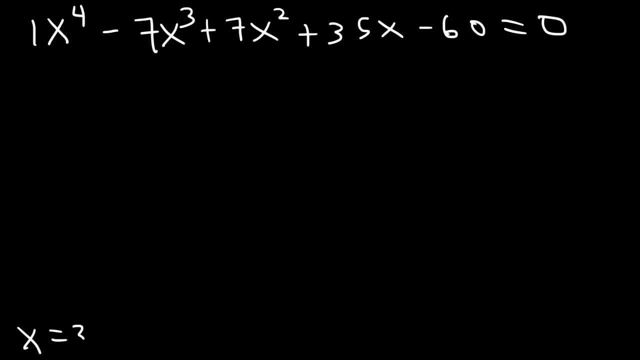 So that's one of the answers. Now let's use synthetic division to find the other ones. So the coefficients are 1, negative 7, 7, 35, and negative 60. So let's bring down the 1.. 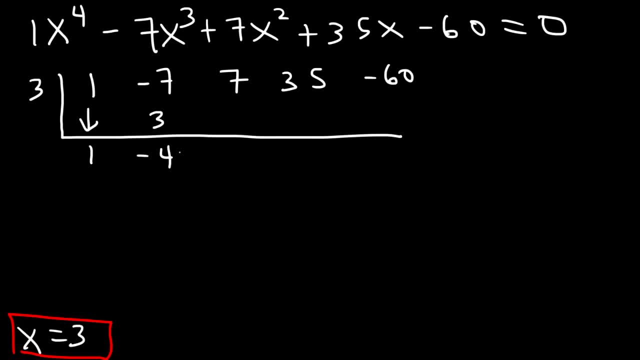 3 times 1 is 3.. Negative: 7 plus 3 is negative 4.. 3 times negative: 4 is negative, 12.. 7 plus negative: 12 is negative, 5.. 3 times negative: 5 is negative, 15.. 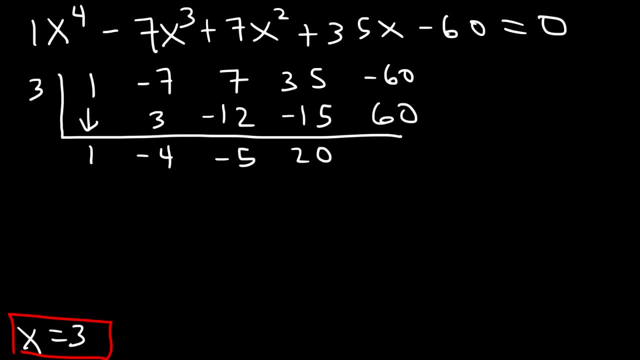 35 minus 15 is 20. And 3 times 20 is 60. So if you get a 0, that's a good sign. So we started with degree 4.. Now it's going to be a degree 3 function. 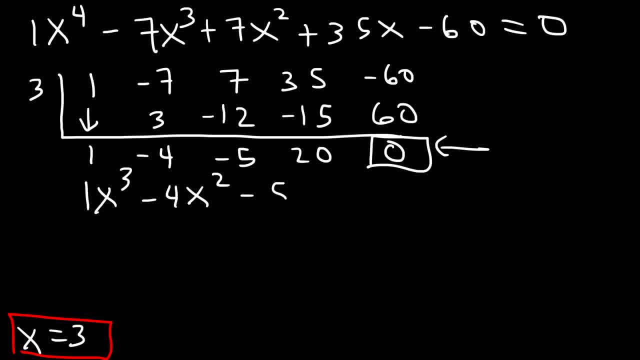 So it's X cubed minus 4X squared minus 5X plus 20.. So notice that we can factor by grouping Negative: 4 divided by 1 is negative 4.. 20 divided by negative 5 is also negative 4.. 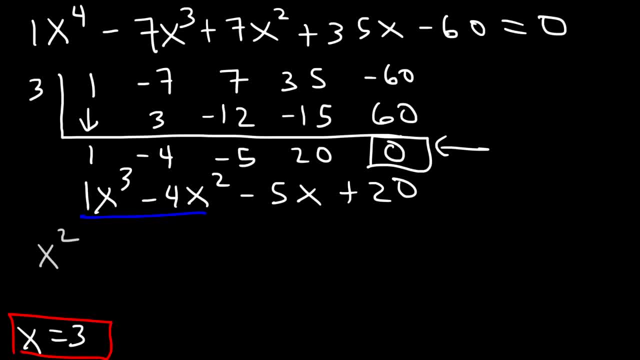 So let's take out the GCF, which is going to be X squared. So X cubed divided by X squared is X Negative. 4X squared divided by X squared is negative 4.. And then let's take out a negative 5.. 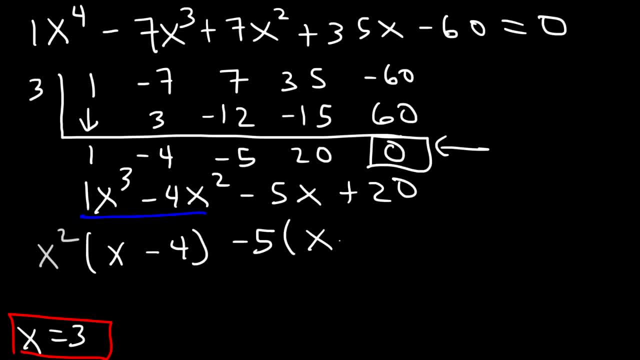 Negative 5X. divided by negative 5 is X. 20 divided by negative 5 is negative 4.. So it's going to be X minus 4 times negative 4.. Times X squared minus 5. And all of that is equal to 0.. 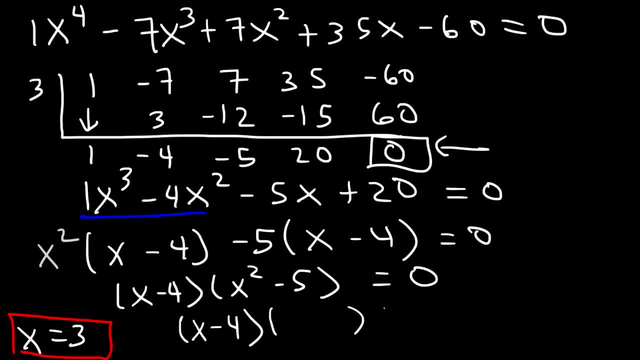 Now let's factor X squared minus 5 using the difference of perfect squares technique, So the square root of X squared is X, The square root of 5 is the square root of 5., And so there's going to be 4 answers in total. 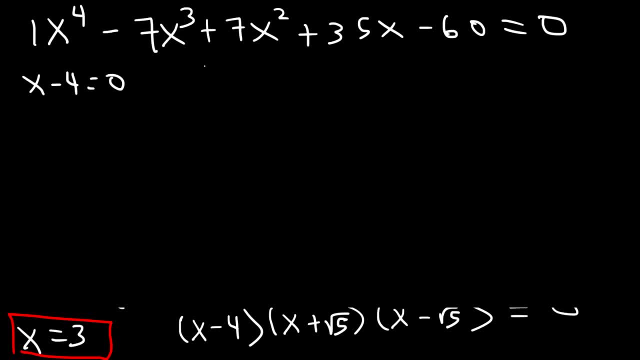 So we could set X minus 4 equal to 0.. X plus the square root of 5 equal to 0.. And X minus the square root of 5 equal to 0.. So X is equal to 4.. Negative square root of 5.. 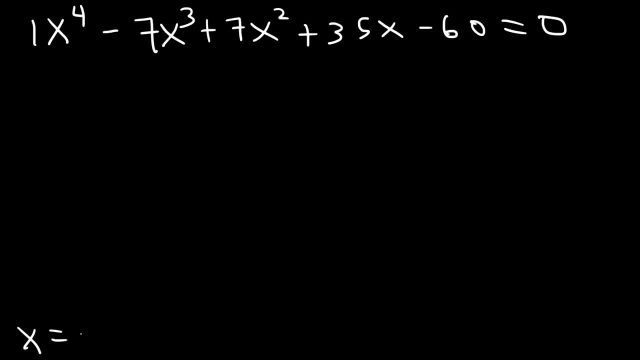 So that's what we're going to do. That's one of the answers. Now let's use synthetic division to find the other ones. So the coefficients are 1, negative 7,, 7, 35, and negative 60.. 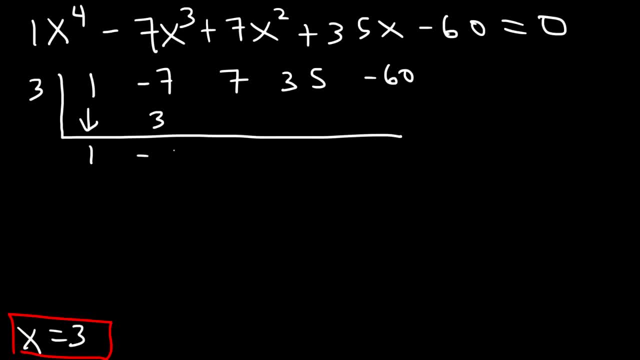 So let's bring down the 1.. 3 times 1 is 3.. Negative: 7 plus 3 is negative: 4.. 3 times negative: 4 is negative 12.. 7 plus negative: 12 is negative, 5.. 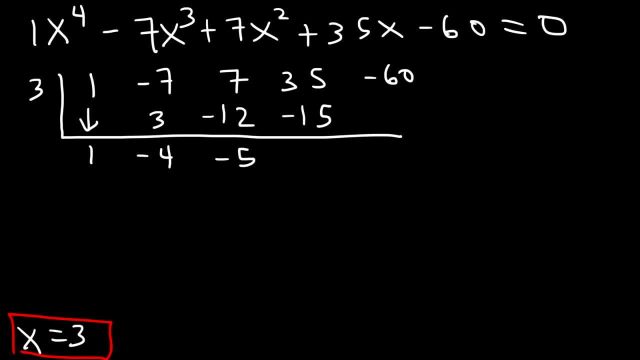 3 times negative, 5 is Negative 15.. 35 minus 15 is 20.. And 3 times 20 is 60. So if you get a 0, that's a good sign. So we started with degree 4.. 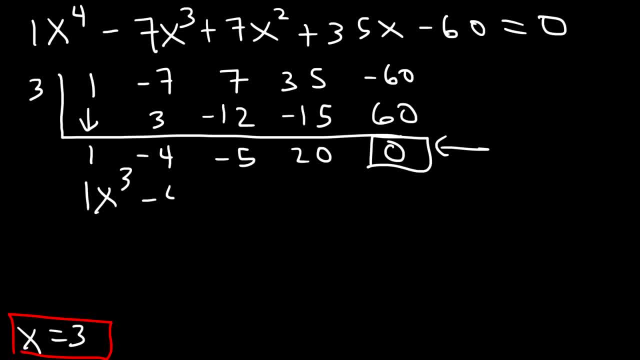 Now it's going to be a degree 3 function, So it's x cubed minus 4x squared minus 5x plus 20.. So notice that we can factor by grouping Negative 4 divided by 1 is negative 4.. 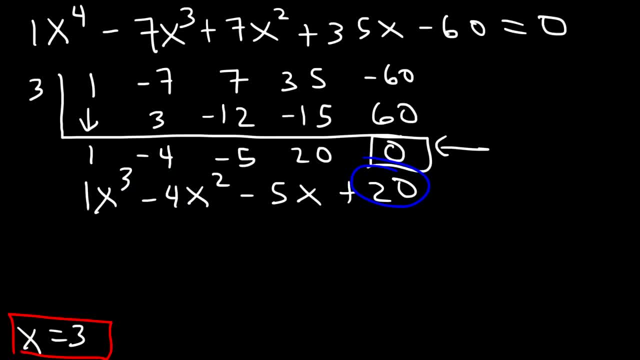 20 divided by negative 5 is also negative 4.. So let's take out the GCF, Which is going to be x squared. So x cubed divided by x squared is x Negative. 4x squared divided by x squared is negative 4.. 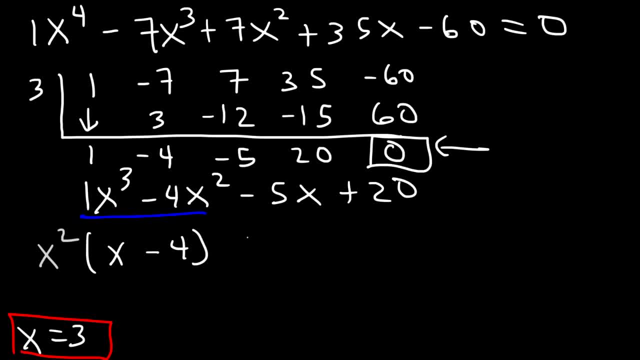 And then let's take out a negative 5.. Negative 5x divided by negative 5 is x 20 divided by negative 5 is negative 4.. So it's going to be x minus 4 times x squared minus 5.. 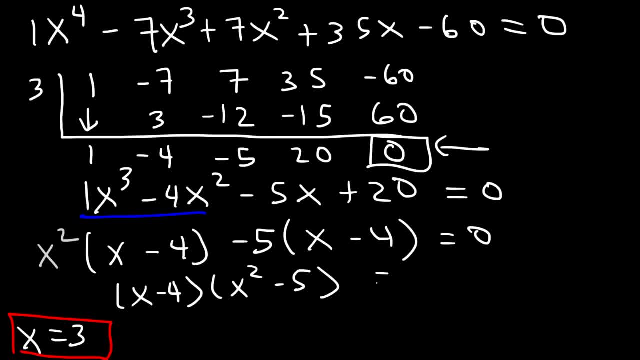 And all of that is equal to 0.. Now let's factor x squared minus 5.. Using the difference of perfect squares technique. So the square root of x squared is x. The square root of 5 is the square root of 5.. 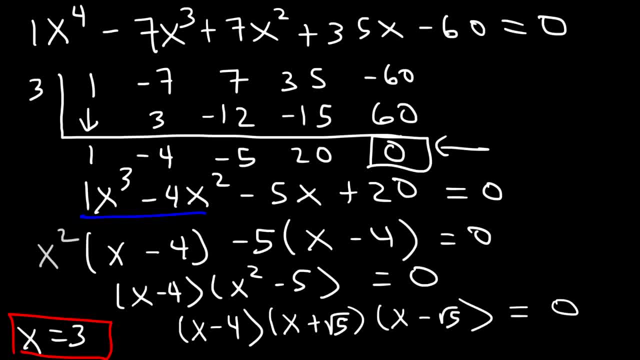 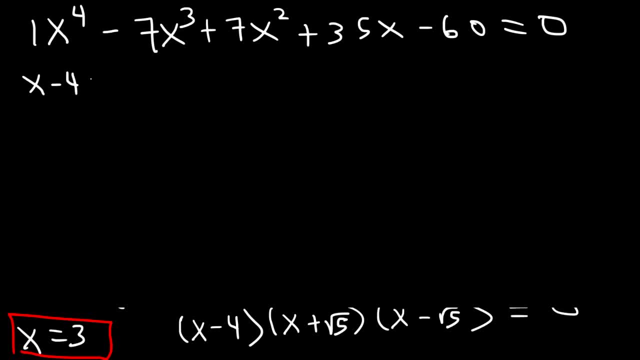 And so there's going to be 4 answers in total. So we could set x minus 4 equal to 0.. x plus the square root of 5 equal to 0.. And x minus the square root of 5 equal to 0.. 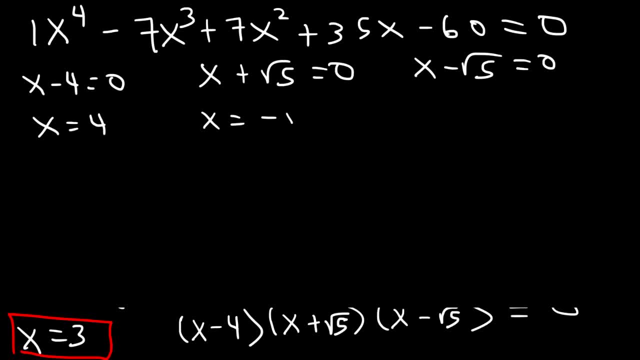 So x is equal to 4.. Negative square root of 5. And positive square root of 5.. So here's the first answer, The second one, The third one And the fourth. So you should have 4 answers for a fourth degree polynomial. 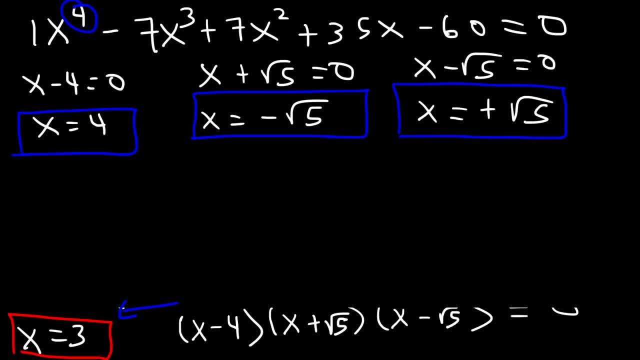 And that's it. So now you know how to solve polynomial equations: By factoring, by grouping, Factoring by substitution And using the rational zero theorem Along with synthetic division. Thanks again for watching. 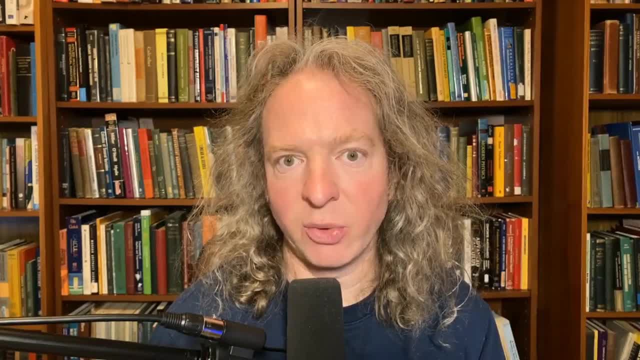 Hello, welcome to another episode of Office Hours with the Math Sorcerer. In today's episode, I'm going to be answering an email I received from a viewer. As always, if you have any advice for this person and you're watching this on YouTube, please leave a comment in the comment section below. If you're listening to this via YouTube or Spotify, you can always come back to 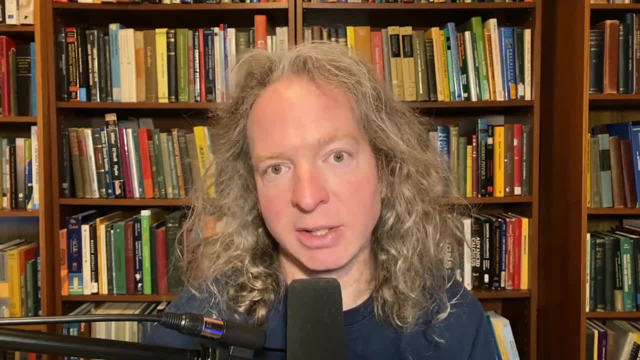 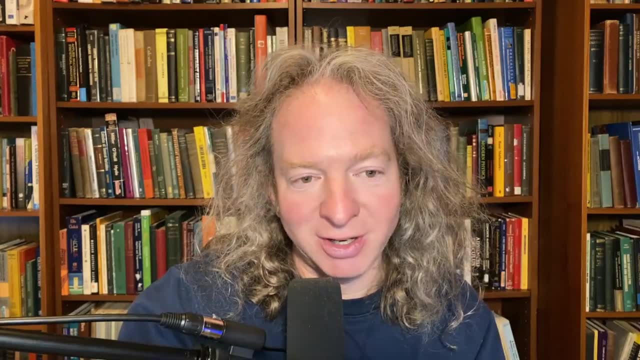 the YouTube video here on the Math Sorcerer YouTube channel and leave your comments. Okay, I'm going to read this email very carefully. It's a little bit longer, but it's actually very interesting. I just said actually. Actually very interesting. I need more coffee. The person's 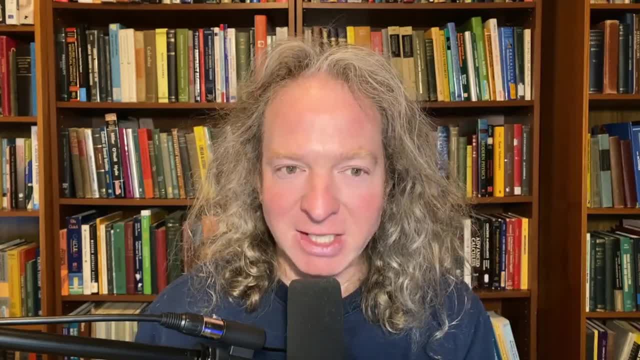 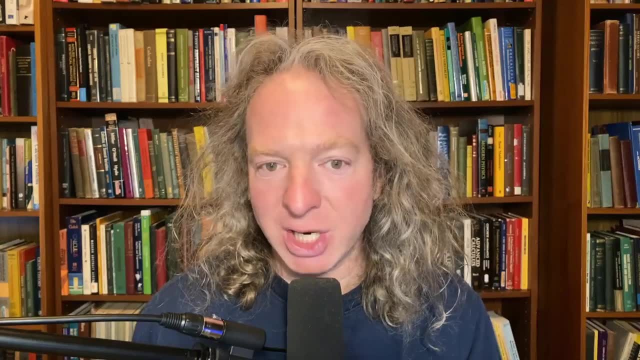 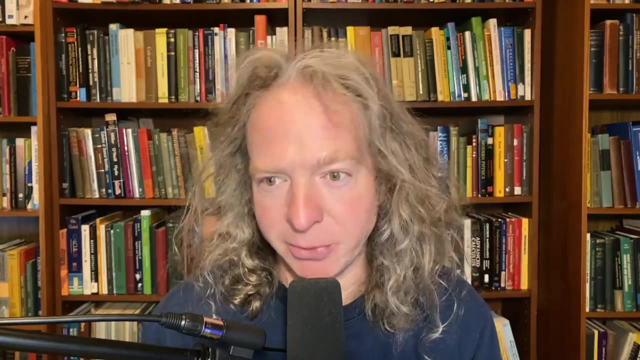 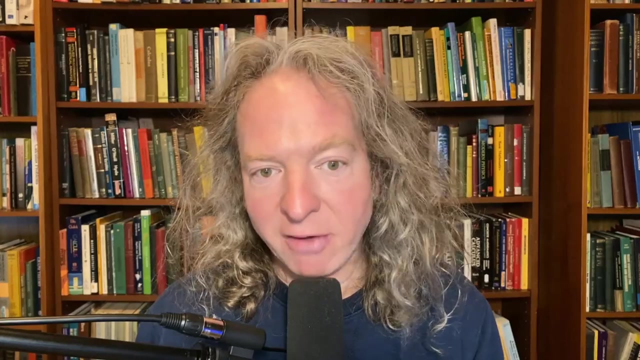 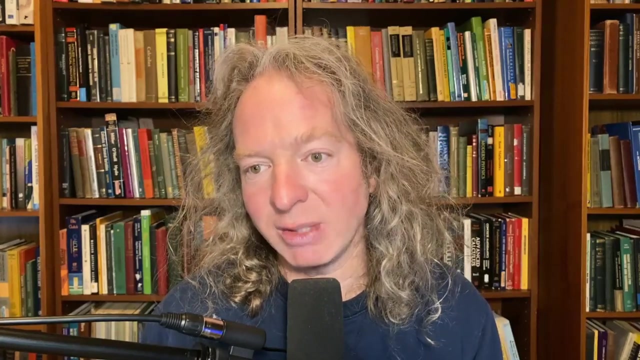 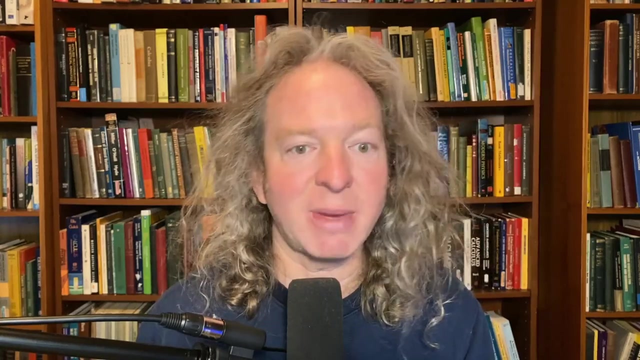 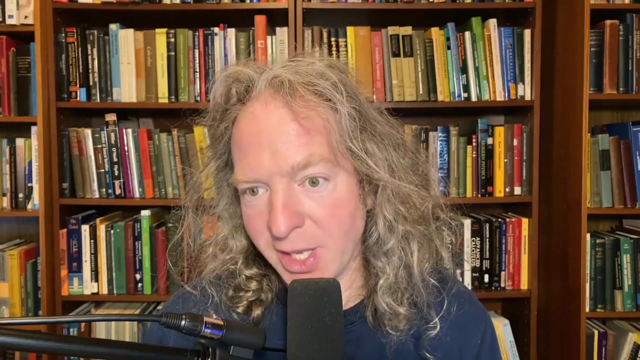 name is Jovan and the subject is advice for med student. Wow. Dear Math Sorcerer, I am a medical student from Croatia and a big fan of your YouTube channel. I enjoy watching your videos and I'm truly grateful for everything you do. I am writing to you to ask you for some advice on how to pursue math in a more formal way. I have always liked math since high school, but I have never had the opportunity to study it at a higher level since math is not really priority in my medical faculty. I was never exceptional at math, but I have always liked doing math and have no problem getting good grades. I have been doing some online exercises from Project Euler and from the YouTube channel Mind Your Decisions, but I want to challenge 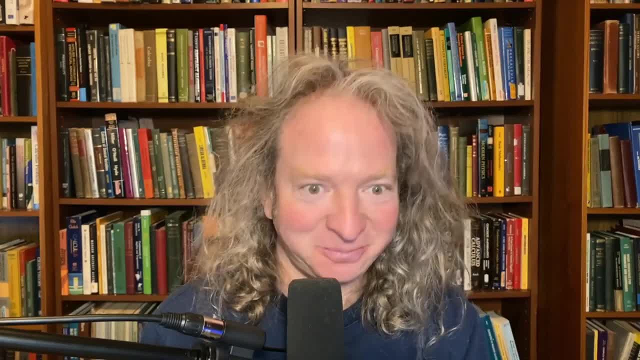 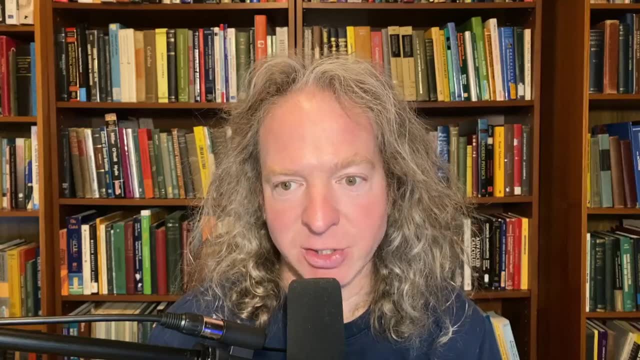 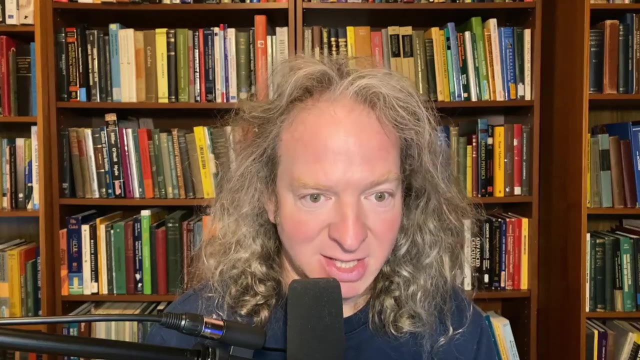 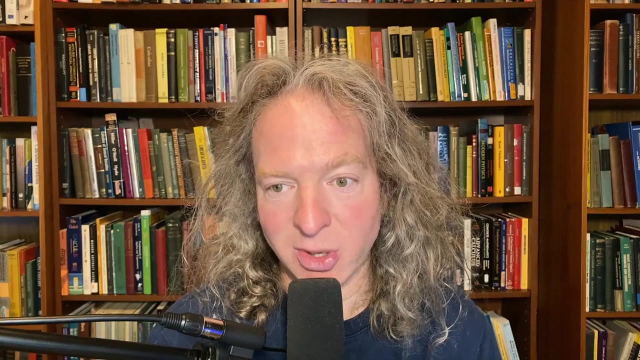 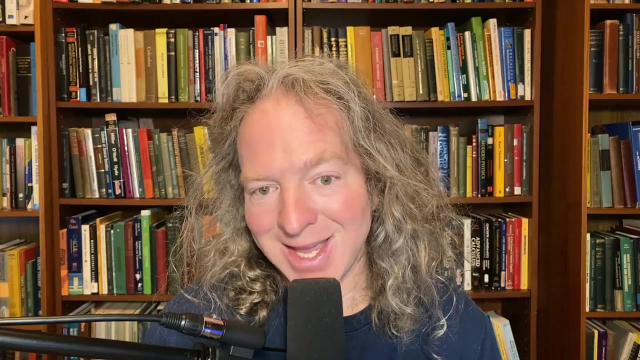 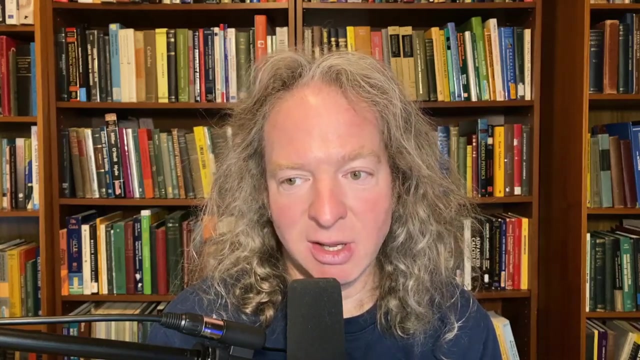 myself more and more. I want to challenge myself more and more. I want to challenge myself more and learn some advanced topics. Okay. I've watched your video where you recommended some huge math books for self-studying math from start to finish. I was very impressed by your collection and your knowledge, but I also felt a bit intimidated by the size. I don't have much time on my hands because of my medical studies, so I was wondering if you could suggest some smaller and more accessible books that are still advanced enough to make me interested or give me some other advice on how to be consistent. I would appreciate any guidance or recommendation you could give me. You are an inspiration to me and many other math enthusiasts. Thank you for your time and attention.